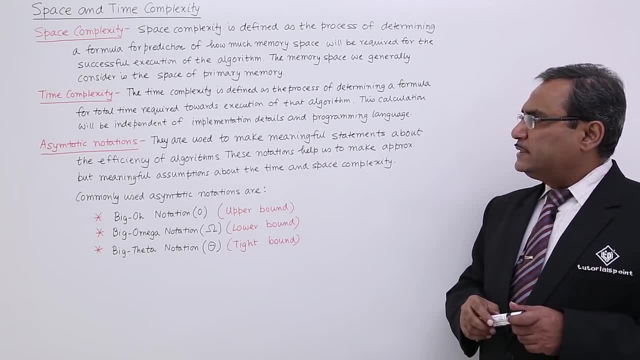 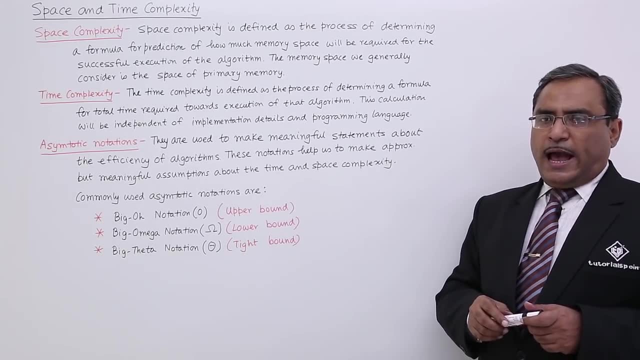 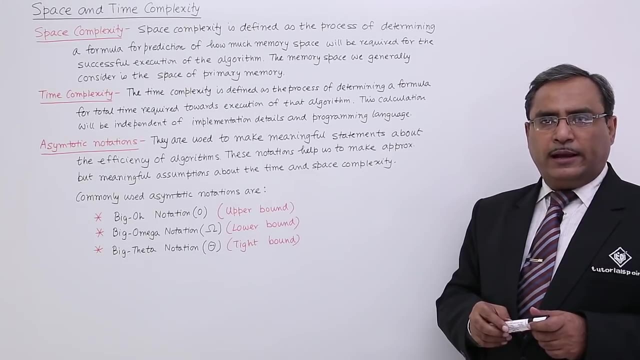 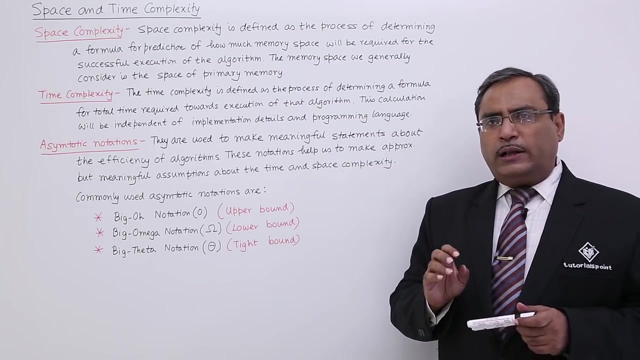 decided in the time complexity. This calculation will be independent of implementation details and, obviously, the programming language. Actually, we are considering the time complexity of an algorithm, So that is why, obviously, it will be irrespective of the programming language selected for the implementation of the algorithm. But simply, if anyone says that, what is the 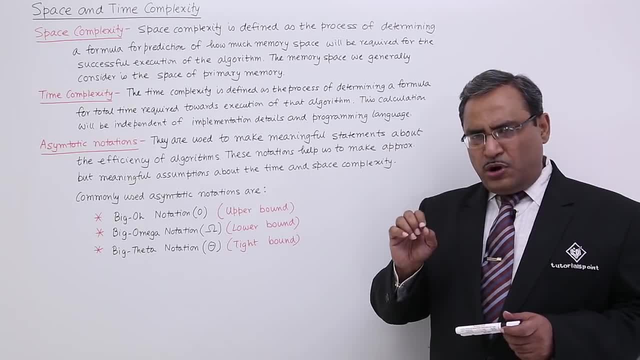 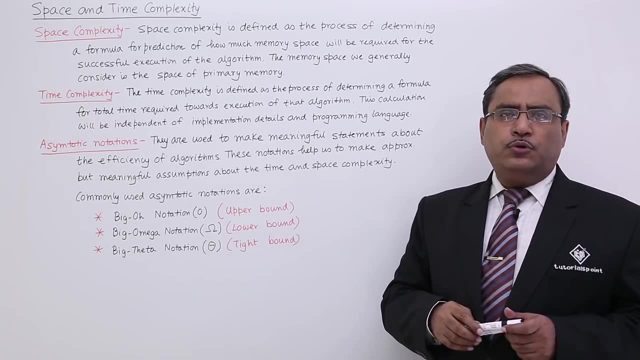 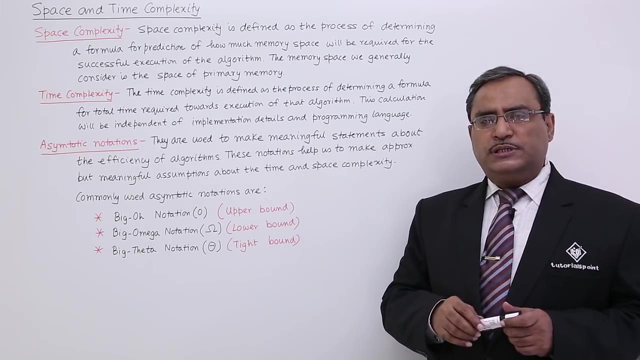 complexity of a program. we commonly consider this as the time complexity. Don't consider the program which will be occupying a very minimum space in the primary memory. That means the program which is having space complexity minimum will be also having the time complexity minimum. 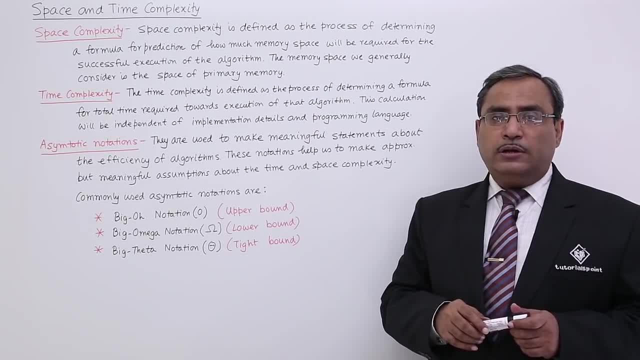 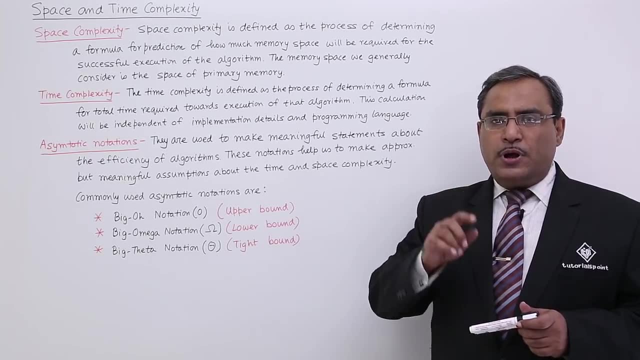 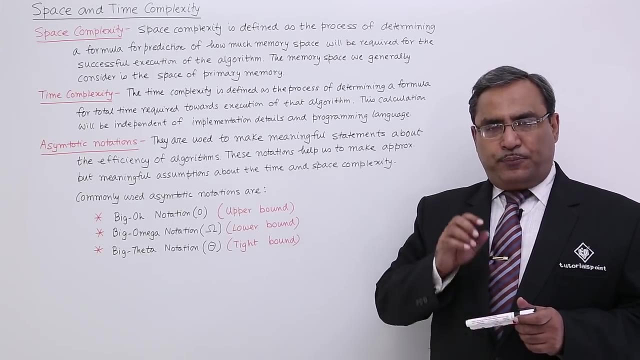 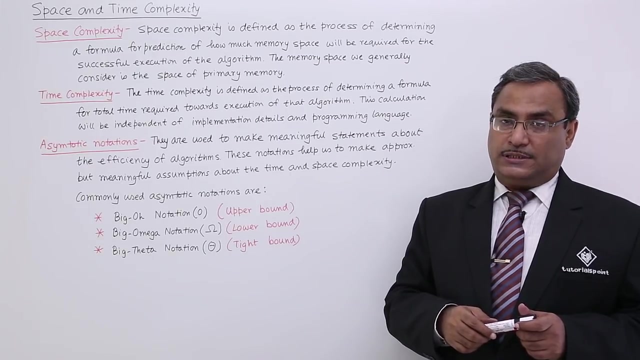 That is not the solution, Because a program might be containing, say, 10 instructions. Out of those 10 instructions, 8 lines are in a loop and the loop will get executed for 100 number of times. Then actually, during the execution, the program is executing 8 into 100 plus 2. That is 802 number of instructions. 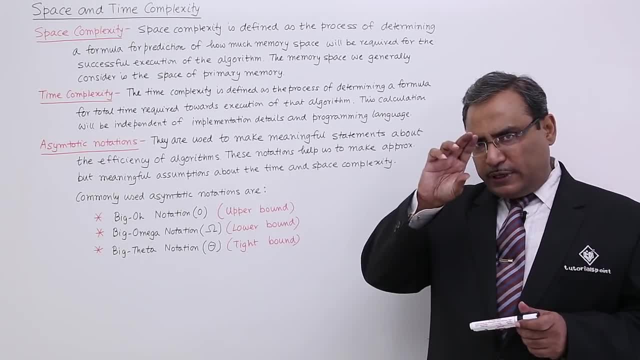 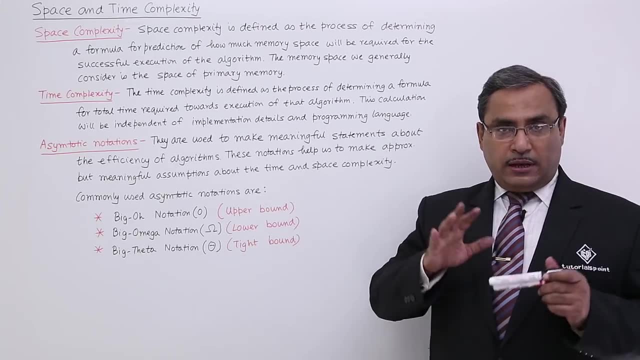 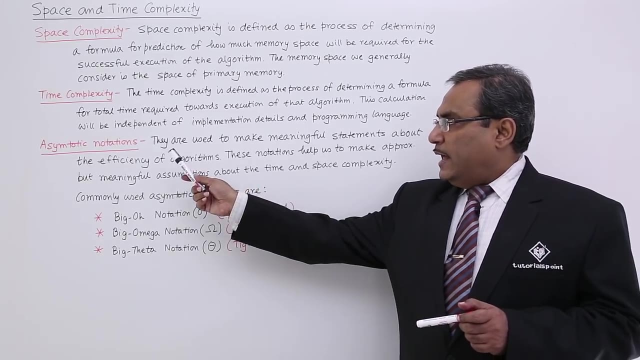 So the memory space has got occupied only for 10 instructions, But during execution it is actually executing 802 instructions approximately whatever calculations I have made right now. So that time complexity of the program will be high. Asymptotic Notations. 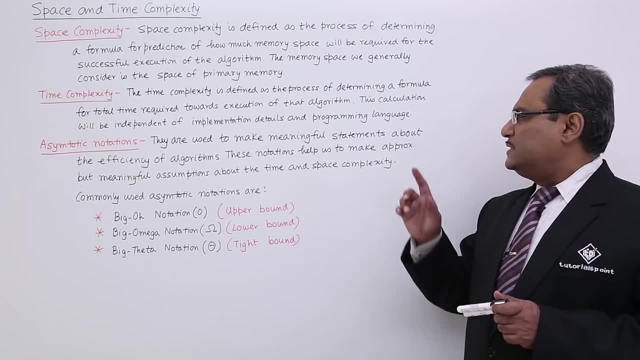 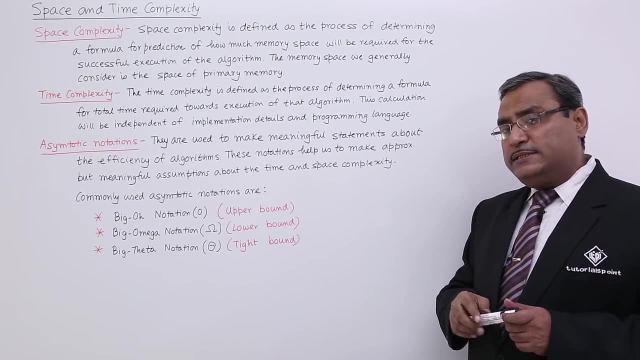 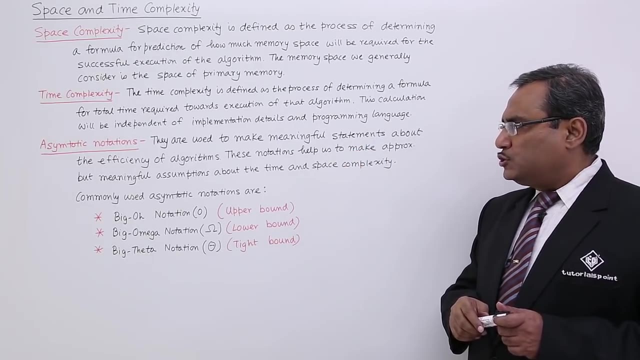 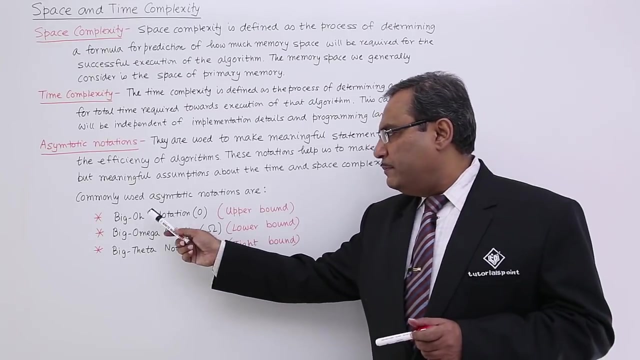 Asymptotic Notations. they are used to make meaningful statements about the efficiency of the algorithms. So they will make some meaningful statements about the efficiency of the algorithm. These notations help us to make approximate manner, As you can see, but meaningful assumptions about the time and the space complexity. So here we are having. 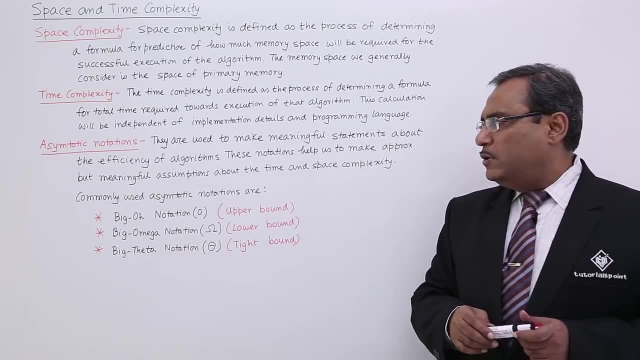 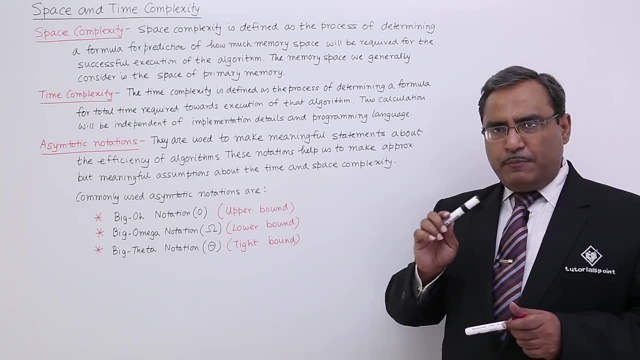 mainly three asymptotic notations. One is the big O notation, So that is a big O, So it is known as the upper bound. That means the maximum complexity. time complexity which will be suffered by this program is known as the will be denoted by the big O notation. 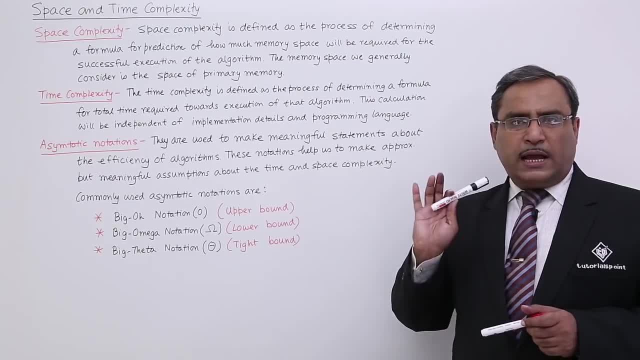 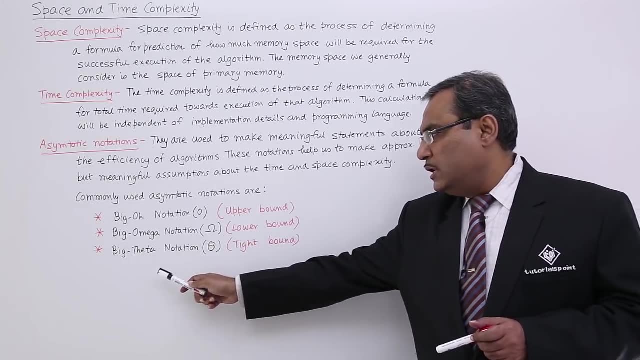 Big omega notation. that is the lower bound, that is the minimum time at least it will take. So that is, the omega will be denoting there is a big omega notation and the last one is a big theta notation will be denoting the tight bound. That means within the upper bound or lower bound. 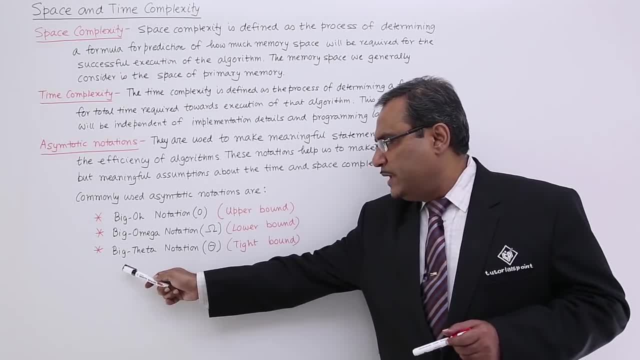 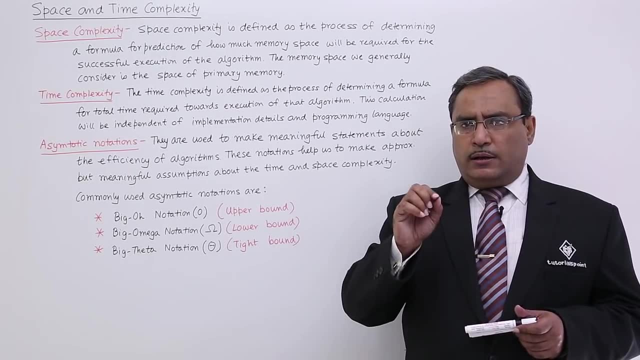 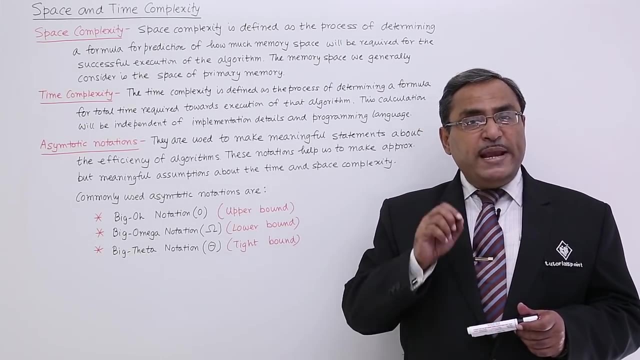 the bound will be mentioned. So that is my big theta notation. Let us suppose we are having n number of data and I am trying to search the one item and to search for one given item value within that set of data, Then what will be the minimum search? 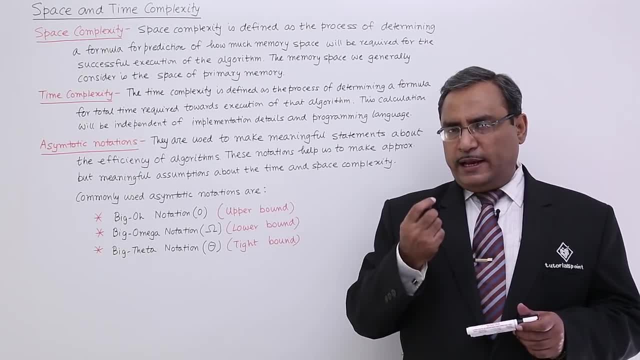 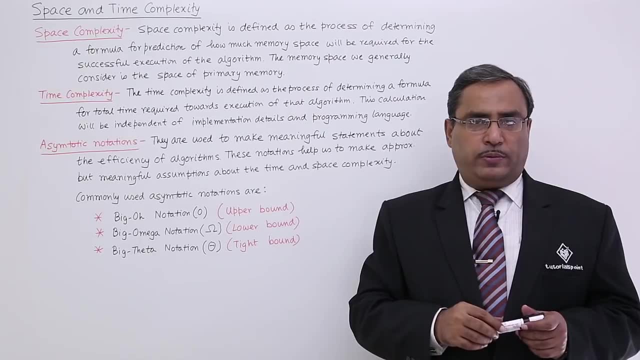 minimum search for the item value. So that is the minimum search for the item value. So number of search required: I think that is one. if I get the search item at the very first place, then I shall say successful completion of the searching. what is the maximum search required so I can find the data at the last, that is. 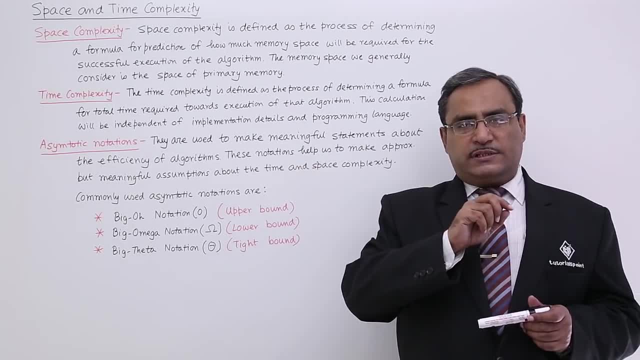 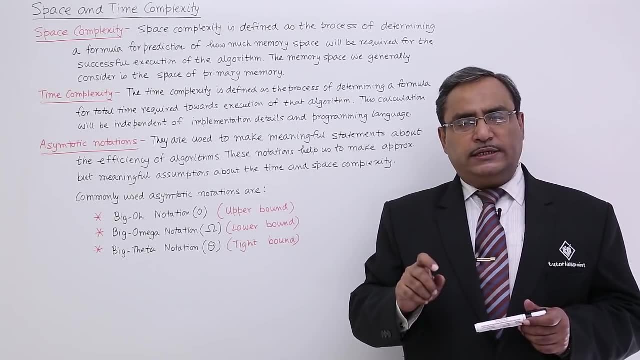 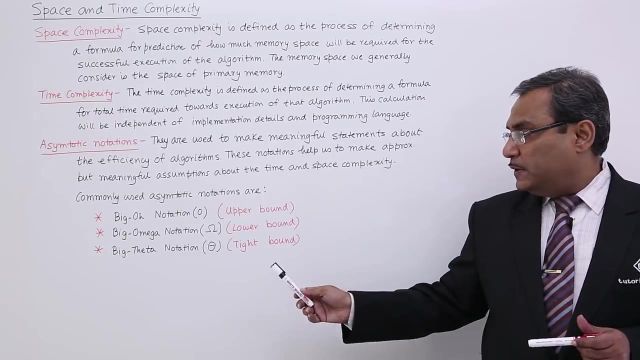 that the nth data will be the search item. otherwise, after searching all n number of data, I am finding that the search item is not there. so in that case, how many searching did I do? n number of searching, and that is the upper bound and what is the lower bound? 1, and in case of tight bound, I can say that we: 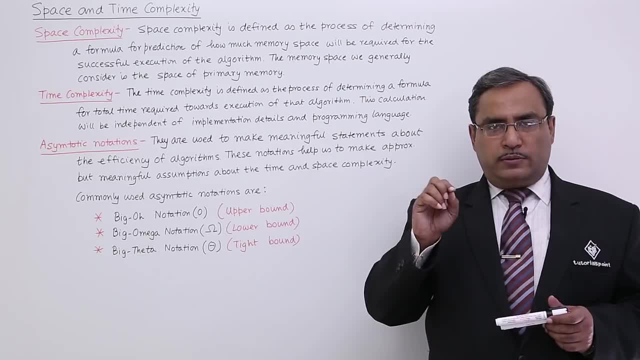 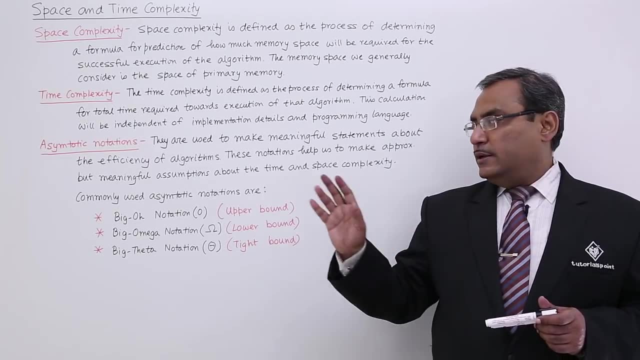 can find this one at the n plus 1, whole by 2 and searching will be required or n by 2. searching will be required if I can get the data at the middle. so that is my. so in case of linear search, the worst case, complexity or the upper bound, will. 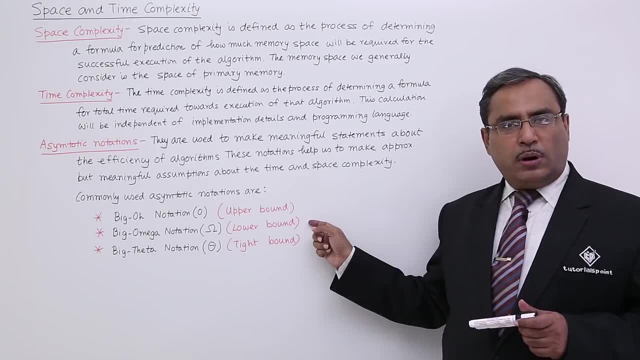 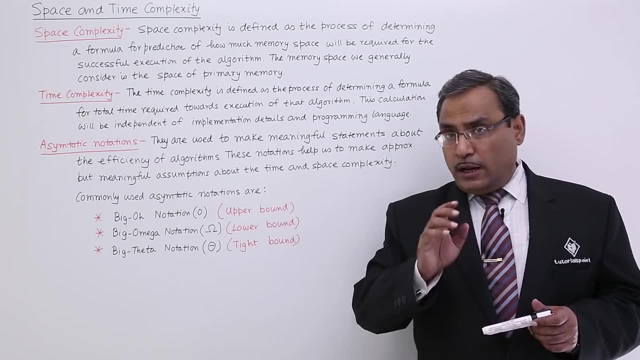 be our n. the best case complexity, or the lower bound, will be our 1, and the average case complexity or tight bound, will be our n by 2. now consider, let us suppose I want to find out the maximum of n number of data in that case just. 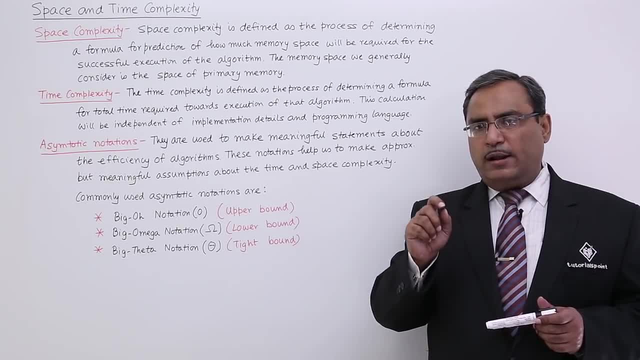 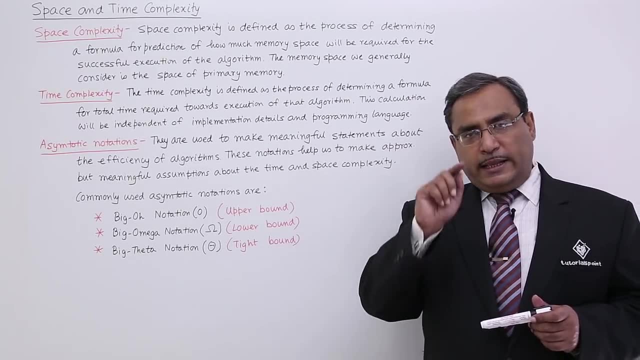 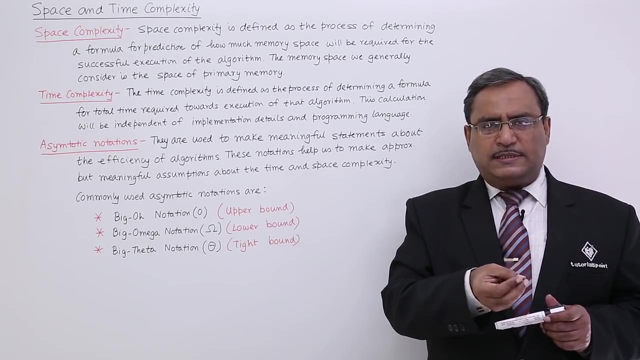 try to fill that to find out the maximum of n number of data you are bound to traverse and compare and process and check all in data. then only you can tell that which is maximum. might be true that the first data which is you are having at the very first place is the maximum, but the maximum is the maximum and the 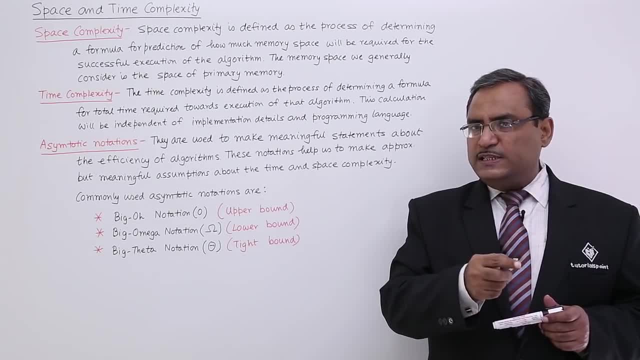 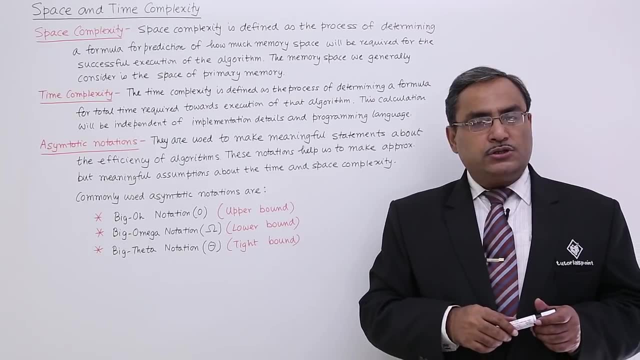 second data is the maximum, but you don't know until and unless that very particular data is being compared with the rest. you cannot tell, you cannot infer, you cannot declare that that is the maximum data. so that means in that case the best case complexity, the average case complexity and the worst.